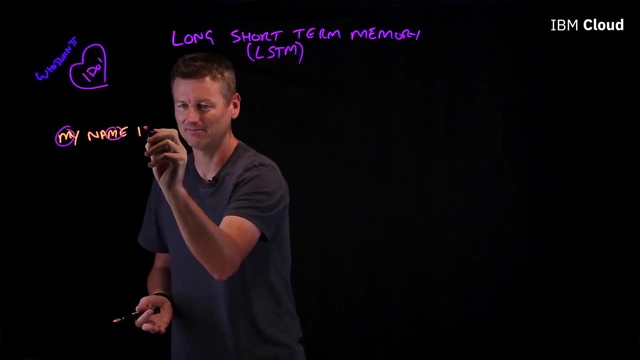 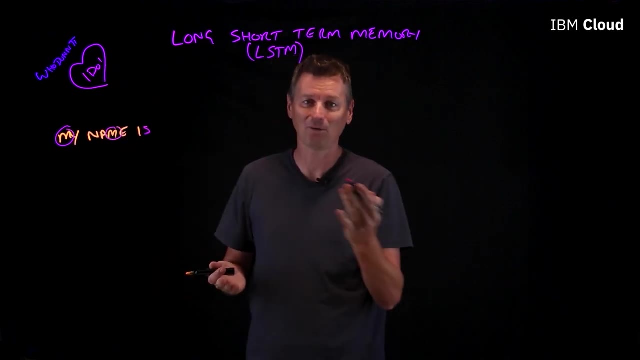 we can establish context and we can clearly see: oh yes, it's my name is. And if we, instead of looking at letters, looked at words, we can establish that the whole sentence here says my name is: oh yes, Martin. 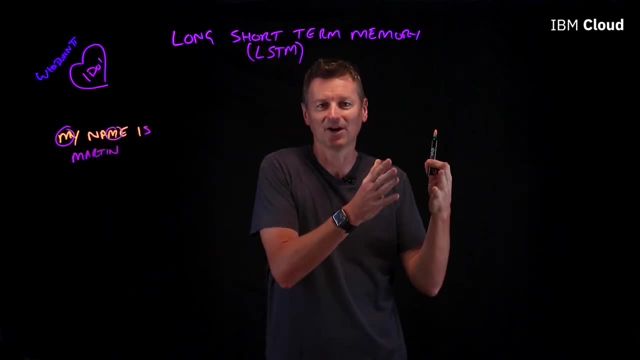 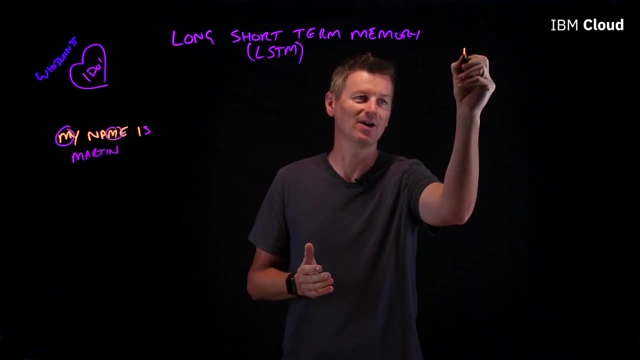 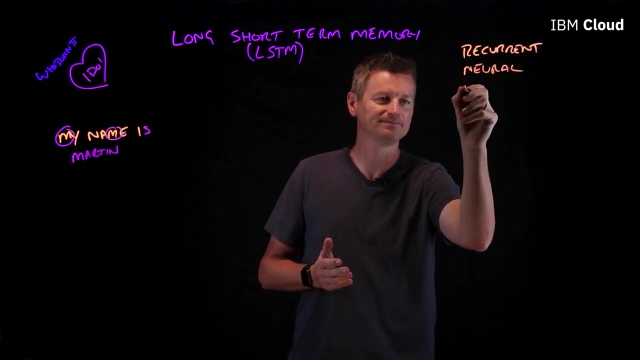 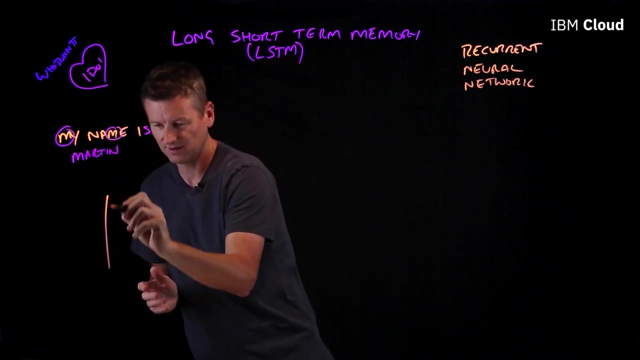 Now, a recurrent neural network is really where an LSTM lives So effectively. an LSTM is a type of recurrent neural network. Recurrent neural net And recurrent neural networks work in the sense that they have a node, So there's a node here and this node receives some input. 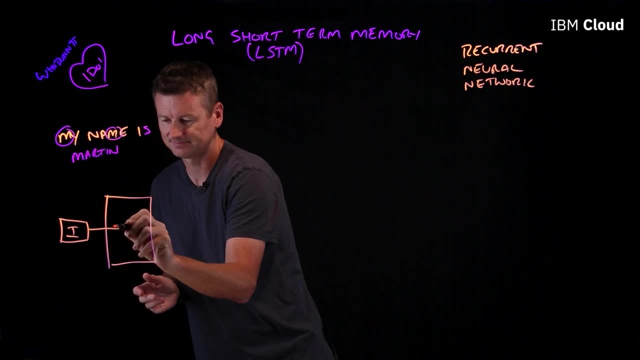 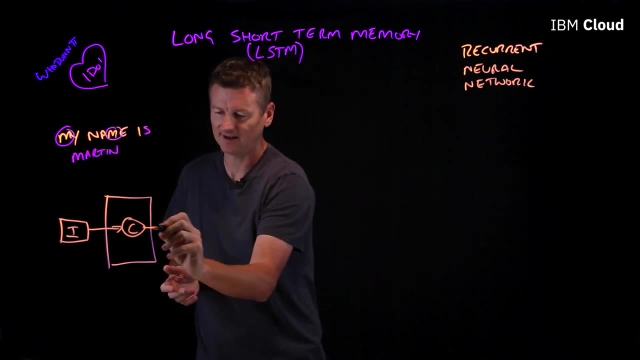 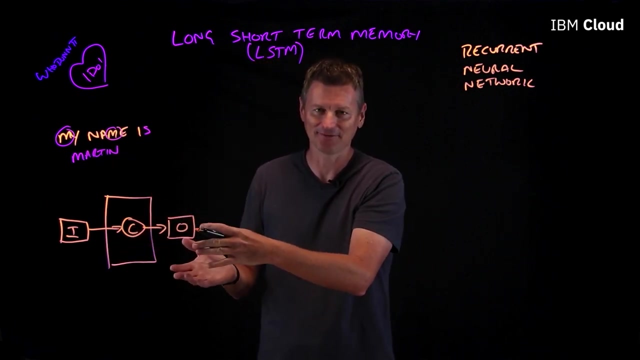 So we've got some input coming in. That input is then processed in some way, So there's some kind of computation and that results in an output. That's pretty standard stuff. But what makes that, What makes an RNN node a little bit different, is the fact that it is recurrent. 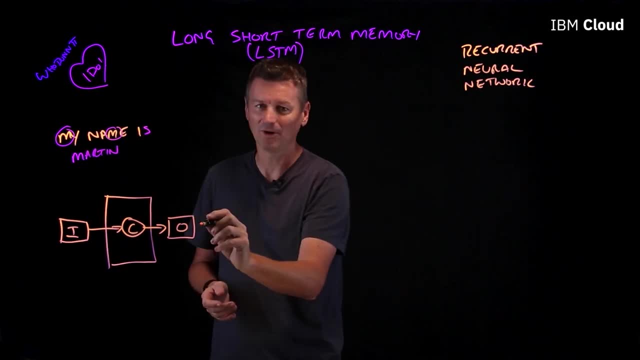 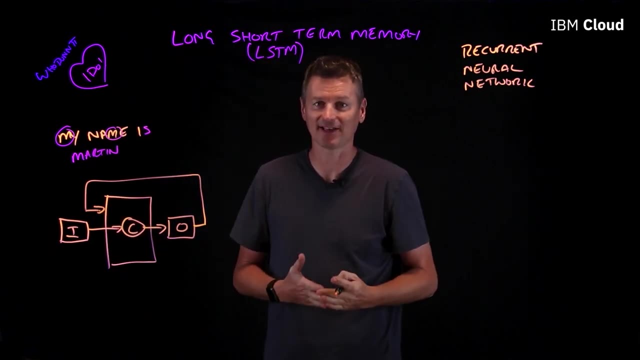 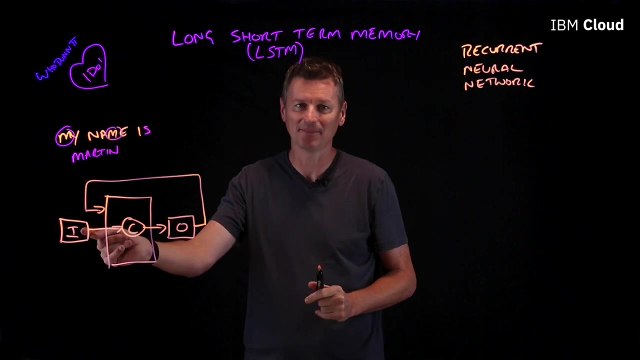 And that means that it loops around. So the output of a given step is provided alongside the input in the next step. So step one has some input, It's processed and that results in some output. Then step two has some new input, but it also receives the output of the prior step as well. 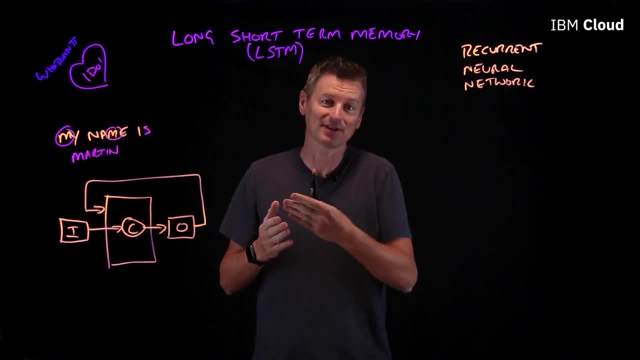 That is what we're looking for. So that makes an RNN a little bit different and it allows it to remember previous steps in a sequence. So when we're looking at a sentence like my name I, we don't have to go back too far through those steps to figure out what the context is. 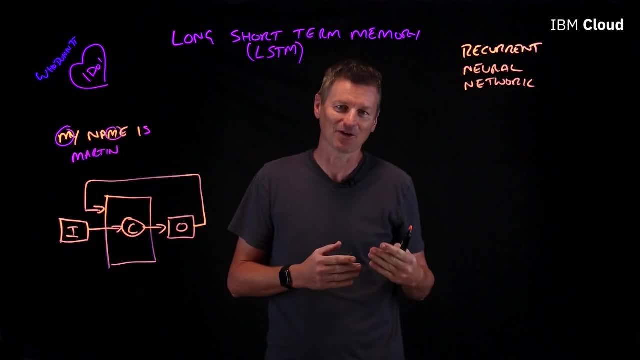 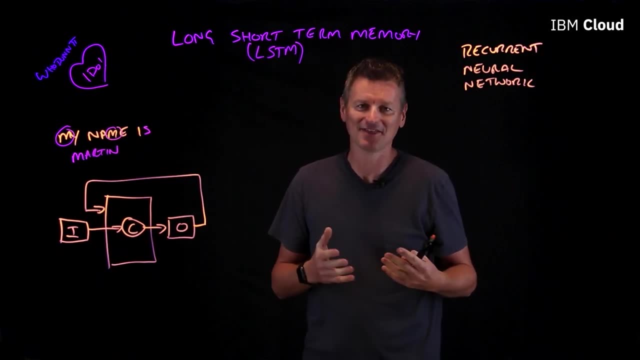 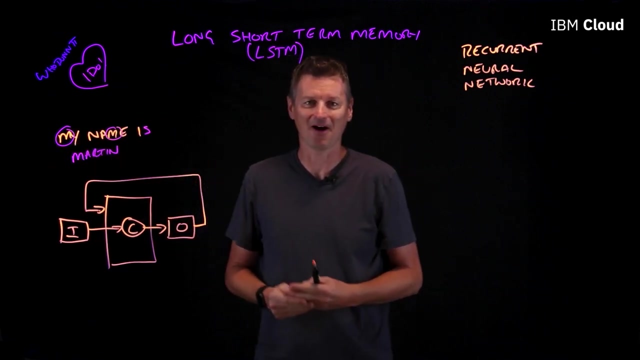 But RNN does suffer from what's known as the long term dependency problem, which is to say that over time, as more and more information piles up, then RNN has become less effective at learning new things. So while we didn't have to go too far back for my name, I, if we were going back through 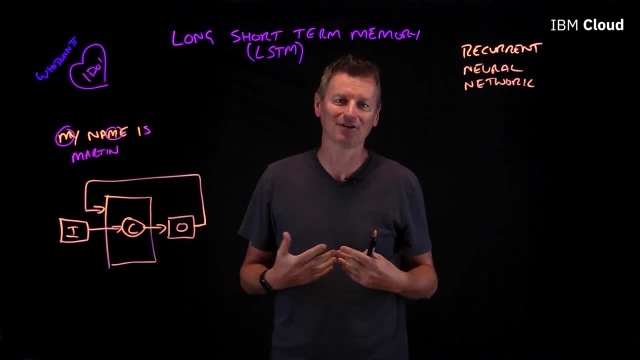 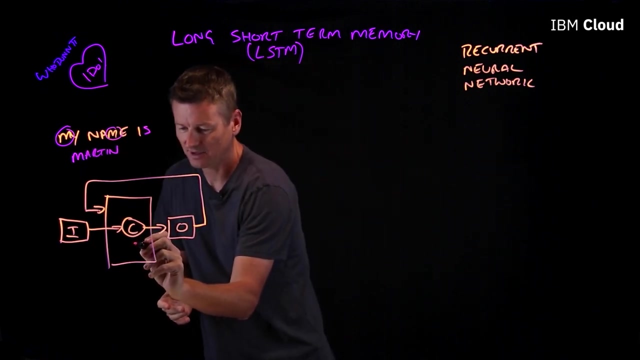 an hour's worth of clues at our murder mystery dinner. well, that's a lot more information that needs to be processed. So the LSTM provides a solution to this long-term dependency problem, and that is to add something called an internal state to the RNN node. 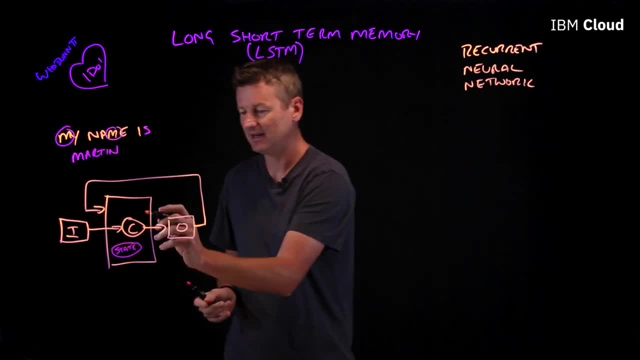 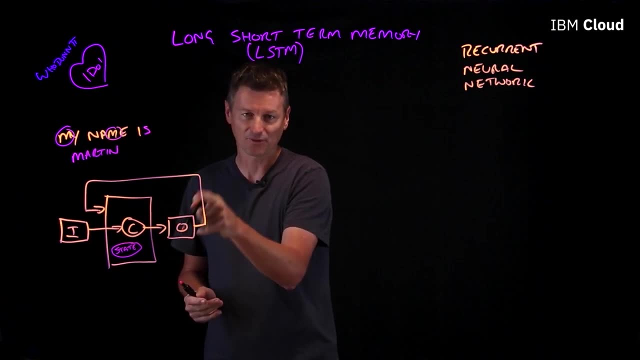 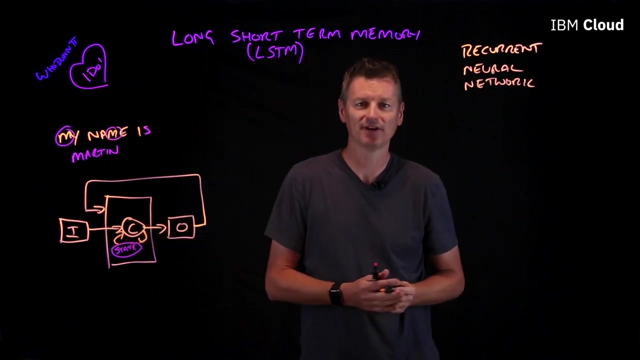 Now, when an RNN input comes in, it is receiving the state information as well. So a step receives the output from the previous step, the input of the new step and also some state information from the LSTM state. Now what is this state? 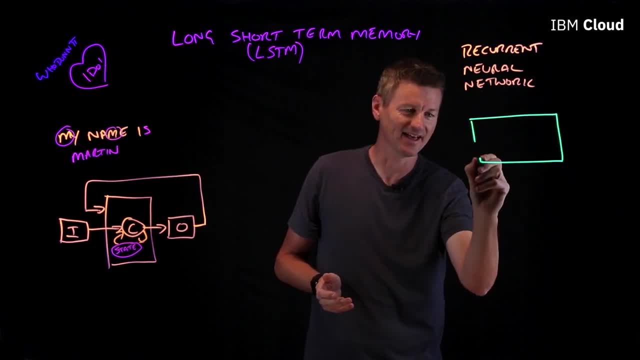 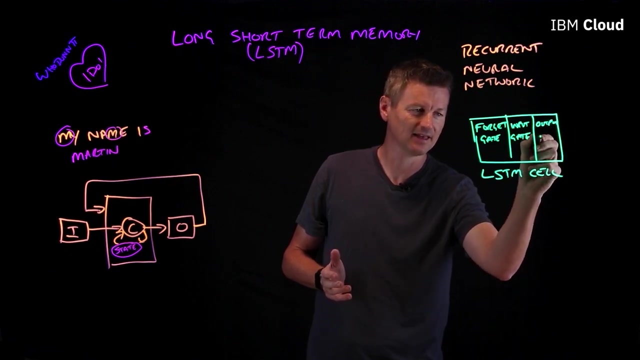 Well, it's actually a cell. Let's take a look at what's in there. So this is an LSTM cell And it consists of three parts. Each part is a gate, There is a forget gate, there's an input gate and there's an output gate. 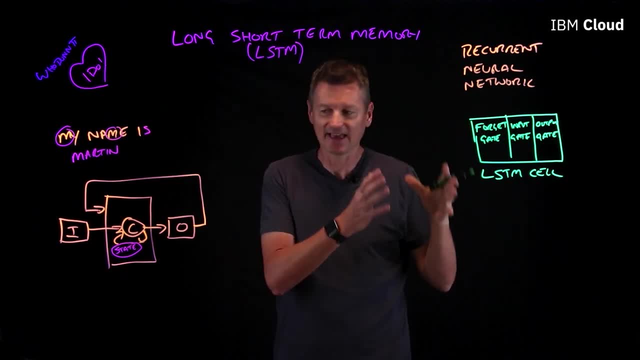 Now the forget gate says what sort of state information that's stored in this internal state here can be forgotten. It's no longer contextually relevant. The input gate says what new information should we add or update into this working storage state information? and the output gate says of all the information that's stored. 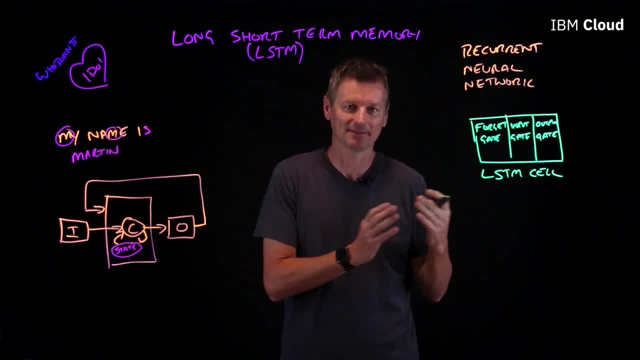 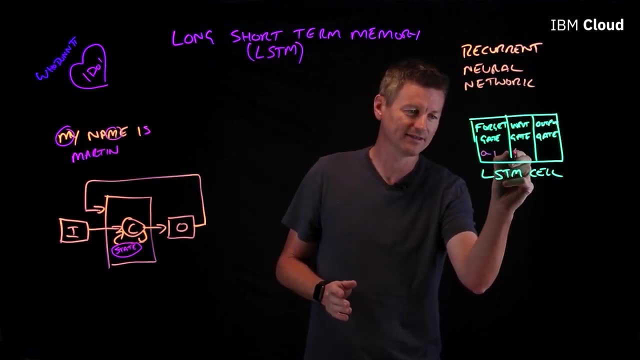 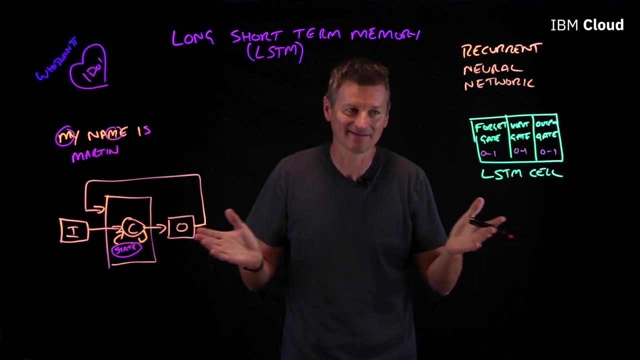 in that state which part of it should be output in this particular instance. And these gates can be assigned numbers between 0 and 1, where 0 means that the gate is effectively closed and nothing gets through and 1 means the gate is wide open. 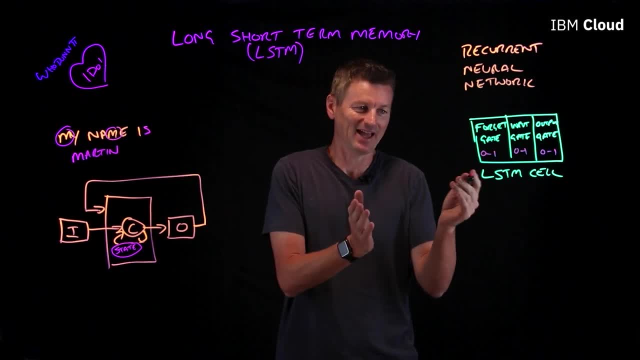 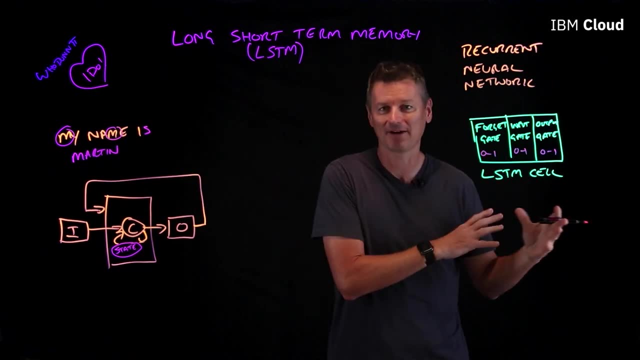 Everything gets through. So we can say forget everything or just forget a little bit. We can say add everything to the input state or add just a little bit. And we can say output everything or just output a little bit, or output nothing at all. 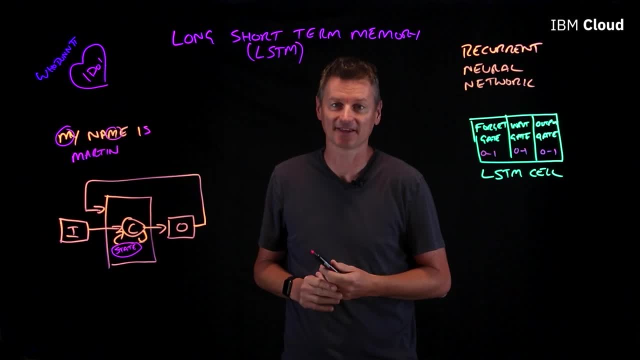 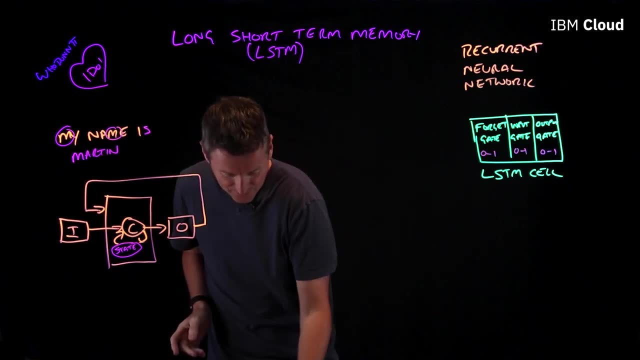 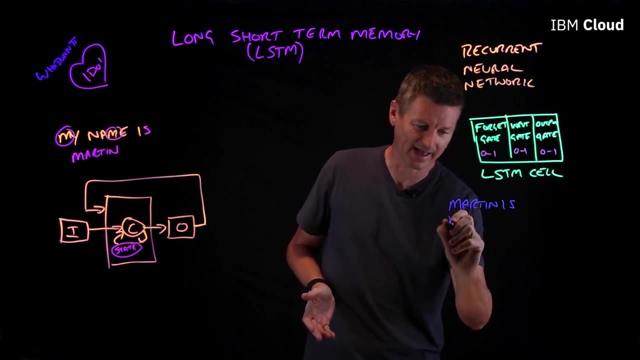 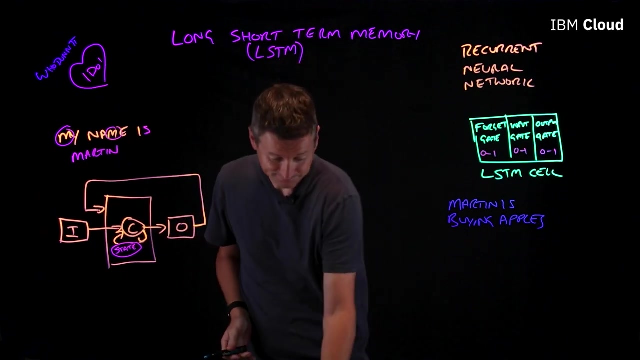 So now, when we're processing in our RNN cell, we have this additional state information that can provide us with some additional context. So if we take an example of another sentence, like Martin, He is buying apples- There's some information that we might want to store in this state. 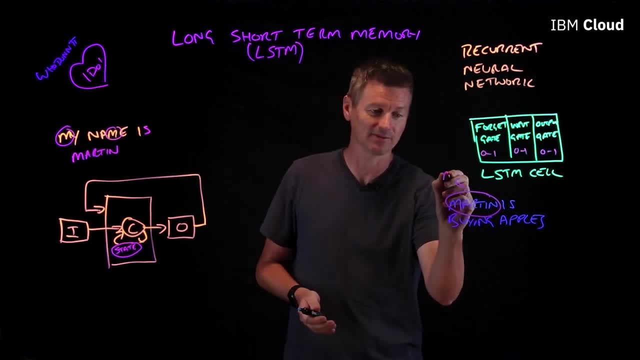 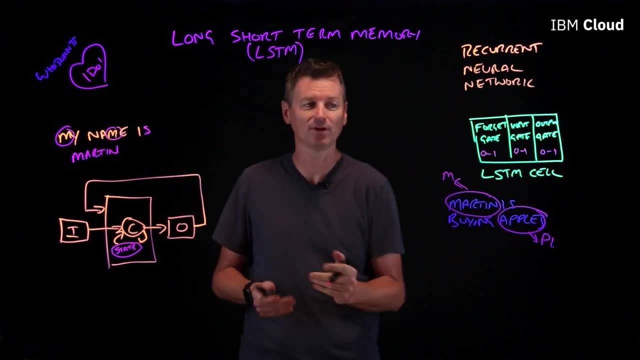 Martin is most likely to derive to the gender of male, so we might want to store that because that might be useful. Apples is a plural, so maybe we're going to store that. it is a plural for later on. Now, as this sentence continues to develop, it now starts to talk about Jennifer.